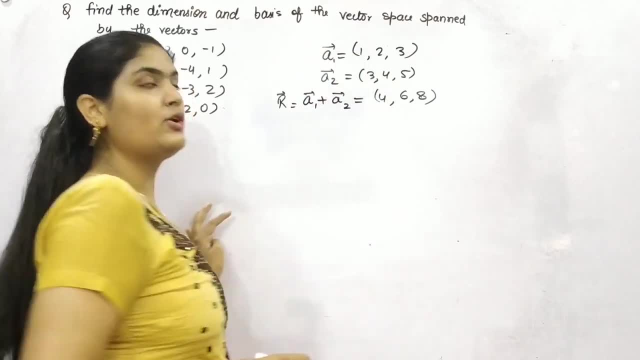 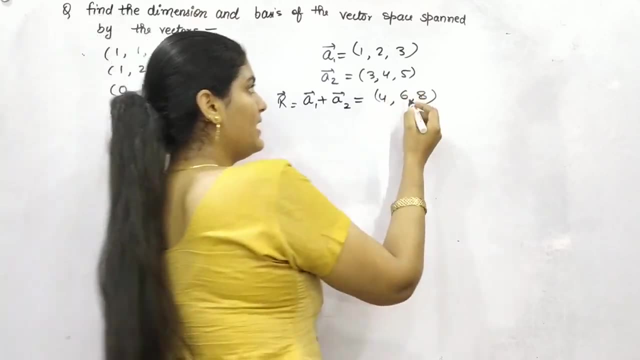 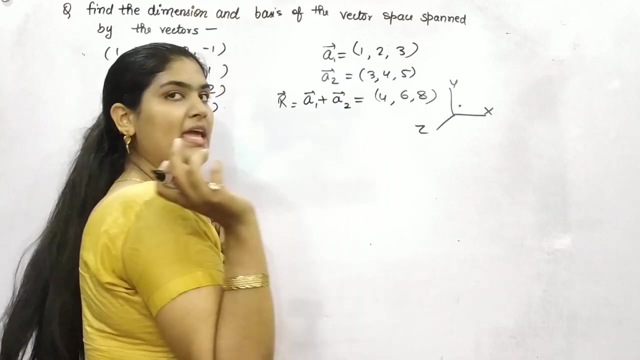 the resulting point is dependent on a1 and a2. That will be counted as linearly dependent. okay, Now you can see. let's say you know x, y and z direction. So let's say any vector space, here a1 and here a2.. 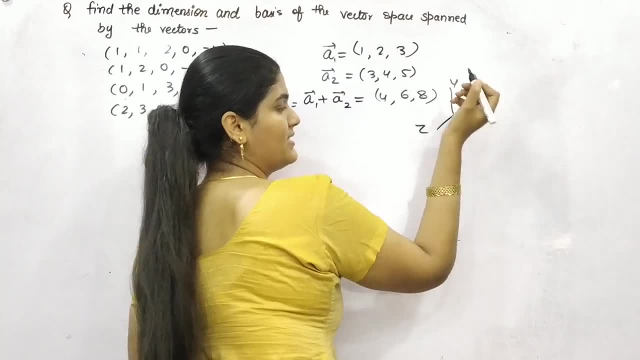 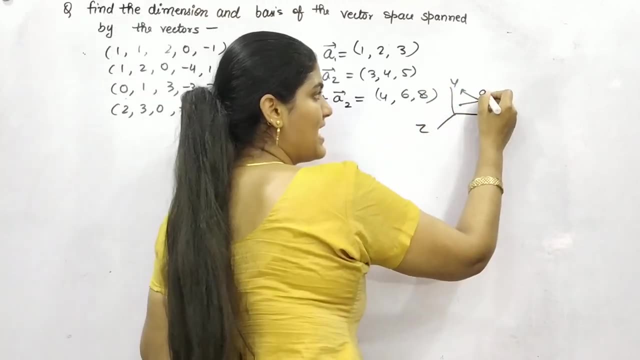 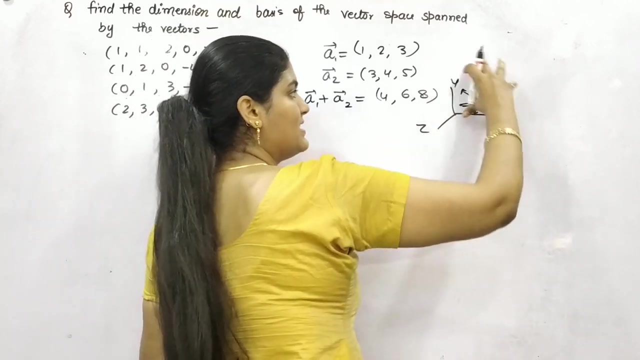 It is moving like this. and it is moving like this. let's say So. the base, which is the base, this is a2.. This is a1 and this is a2.. Base will determine that the origin of these vectors, Whereas these 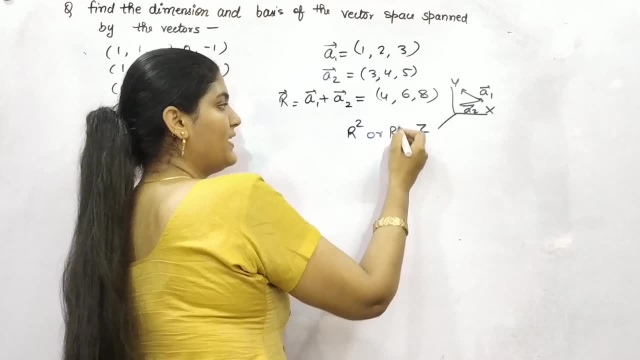 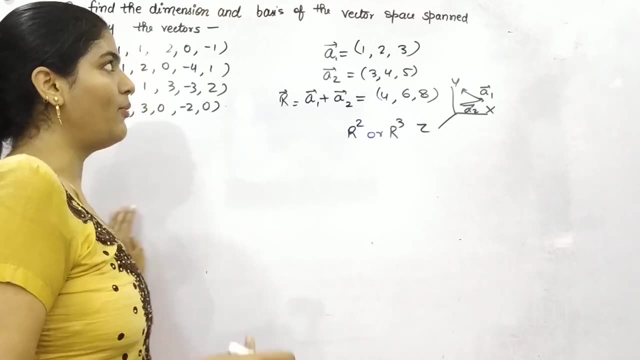 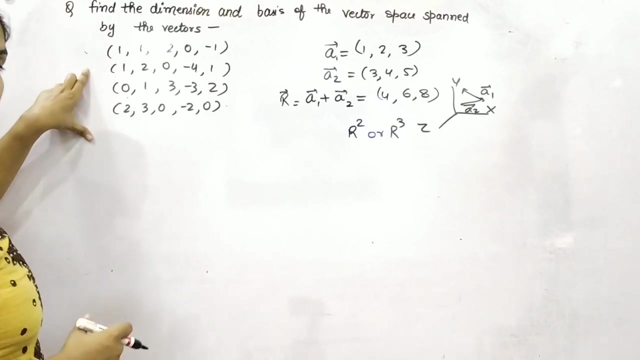 span. whether it is 2D or three dimensional, it will be its dimension. okay, So let's begin with an example: how we can find out a base and dimension of a vector So you can see the span of vector. the vectors are given to you, What you need to do to find out dimension and basis. 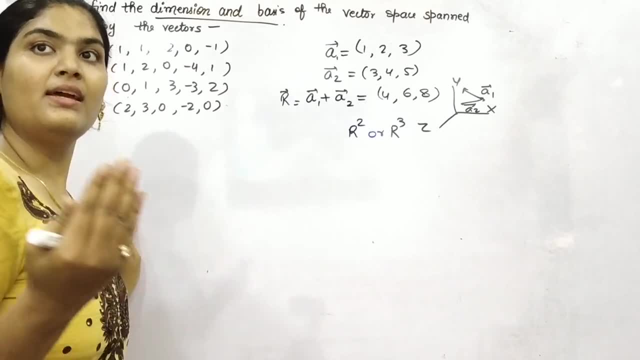 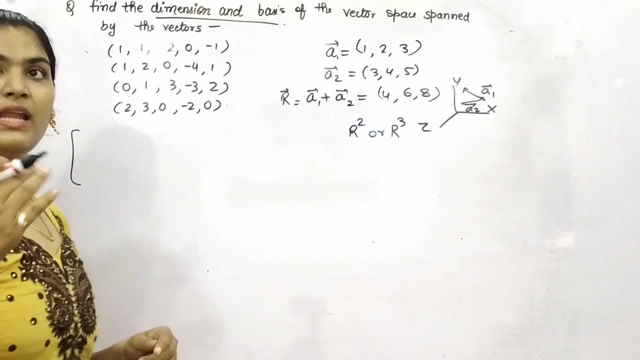 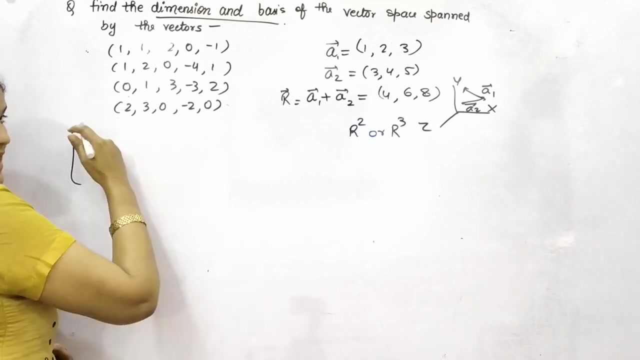 First of all, find out, make a linearly independent matrix. okay, And how you can make it. Let me tell you how You can apply many methods, but I am telling you, with elimination- That is also row elimination- Try to make the elements under the diagonal as 0, okay, So it is 1, 1, minus 2, 0, minus 1.. 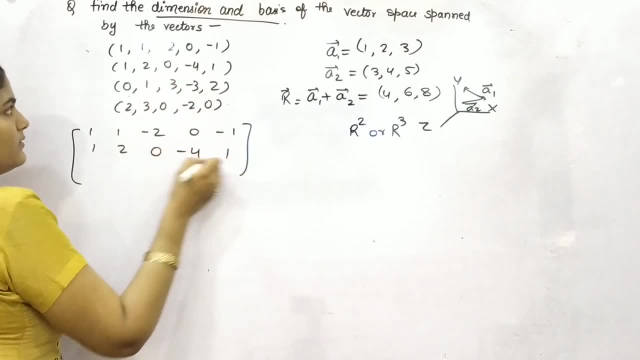 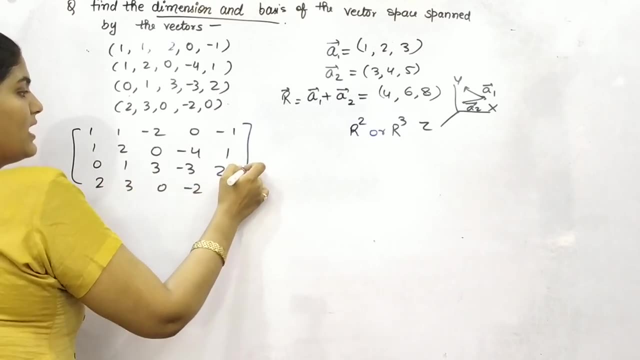 1, 2, 0, minus 4, 1.. 0, 1, 3, minus 3, 2.. 2, 3, 0, minus 2 and 0.. Okay, Now what you need to do. 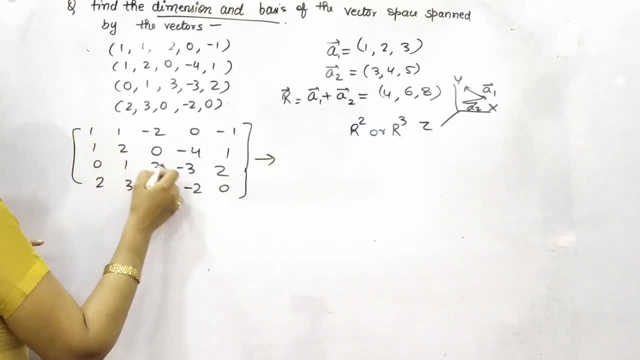 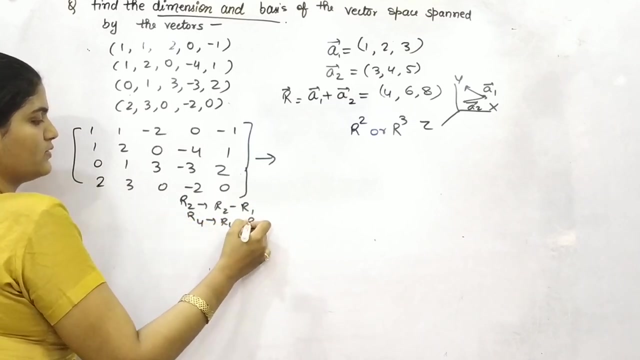 this is 1 already and this is 0. This is your diagonal matrix. Make these things as 0.. Okay, Now you can see what we can apply if we subtract R2 from R1 and for R4 also twice of R1. Then you: 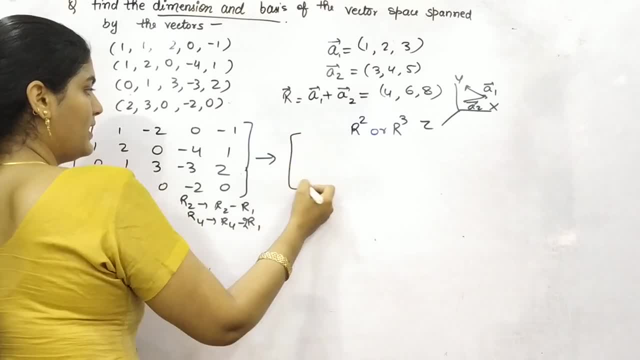 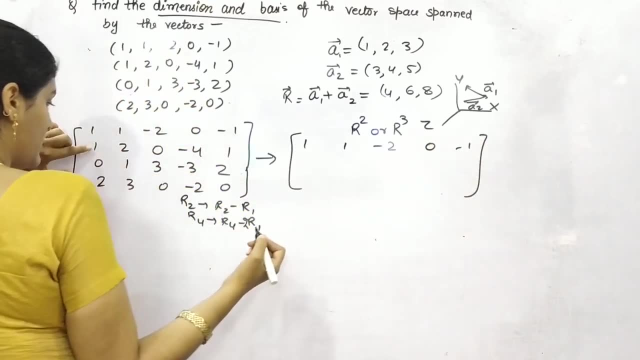 will get 0, right. 2 minus 2 is 0.. So it will be: first is as it is right. Second: R2 minus R1.. 1 minus 1 is 0.. 2 minus 1 is 1.. 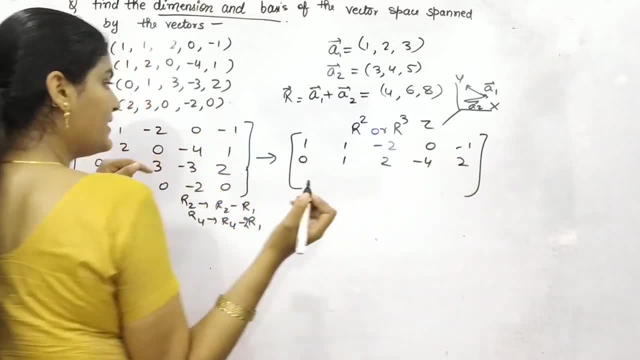 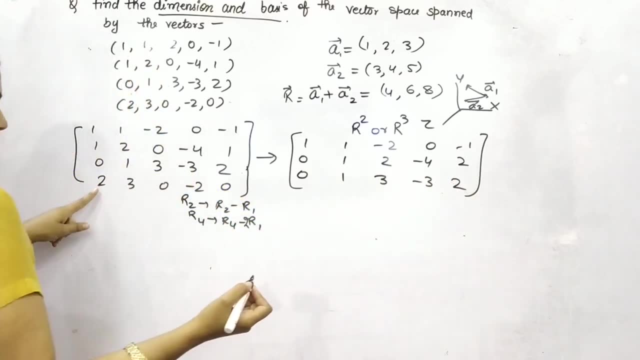 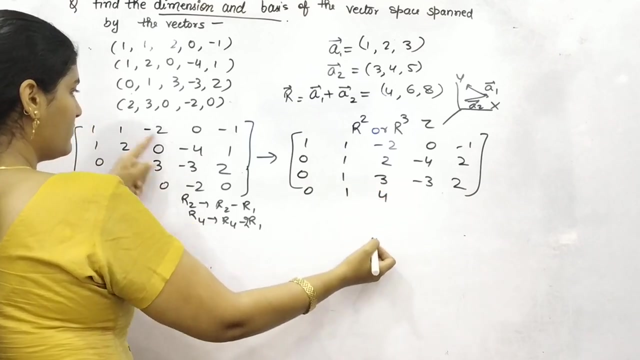 Plus 2 minus 4, 2, right Thereafter this is as same, because we have already got 0 here and R4 minus 2 R1.. So 2 minus 2 is 0.. 3 minus 2 is 1.. Minus minus plus 4, minus 2 and plus 2,. 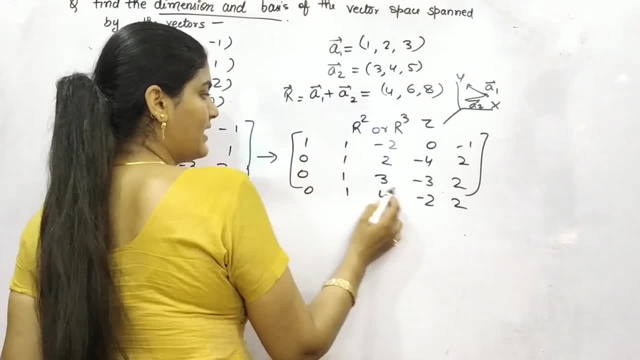 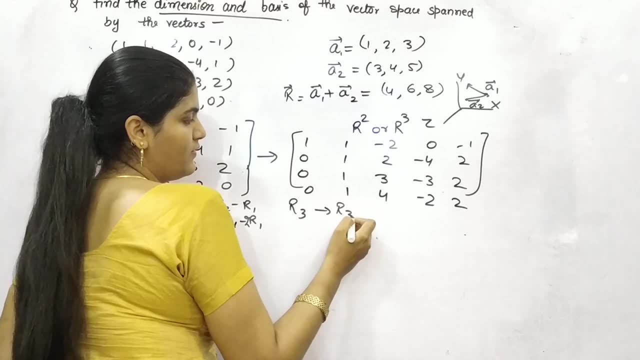 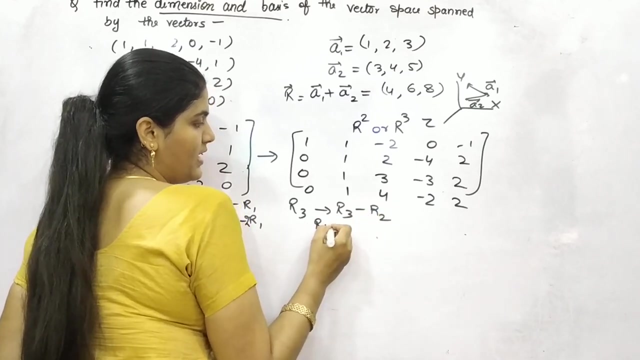 right Thereafter. this is your diagonal matrix, So make this: 0.. R3, if you can subtract R3 from what you can do R3 from R2 and for R4 as well. Okay, So it will become. 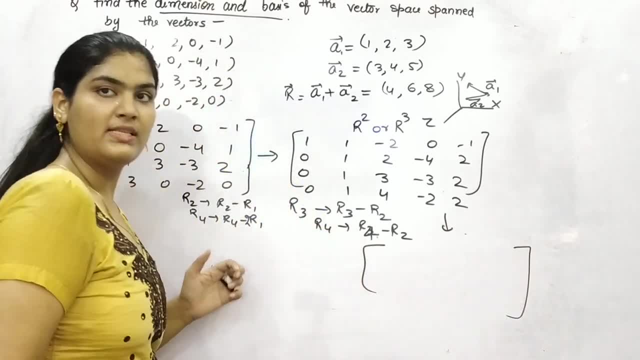 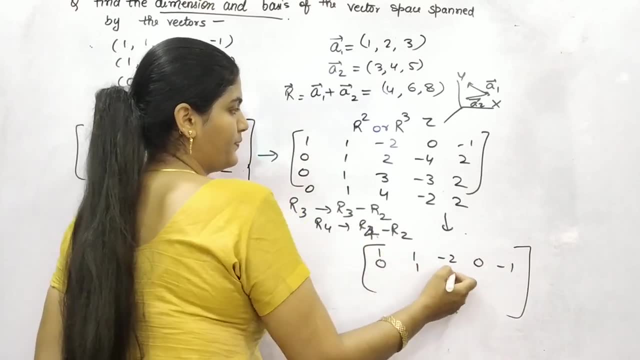 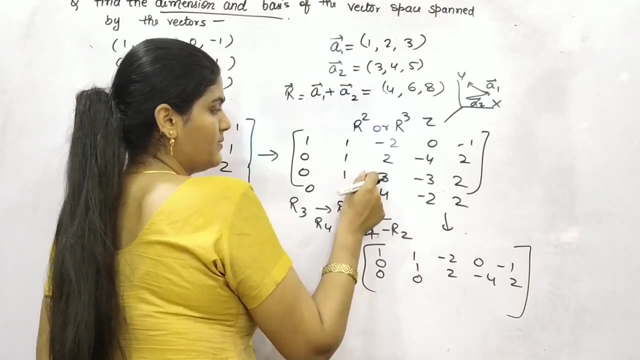 let me do it here, I hope you can see it. So: R1 and R2 same. Then after R3 minus R2, 0 minus 0 is 0, 1 minus 1 is 0, 3 minus 2 is 1. 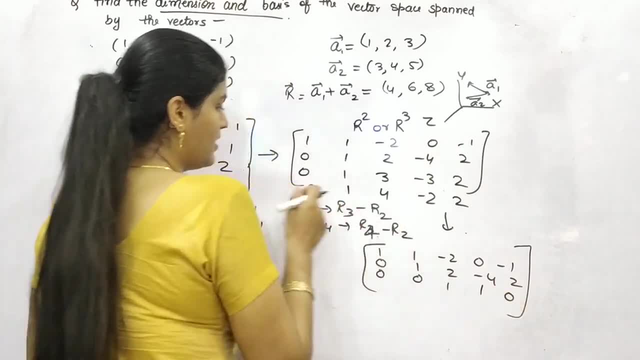 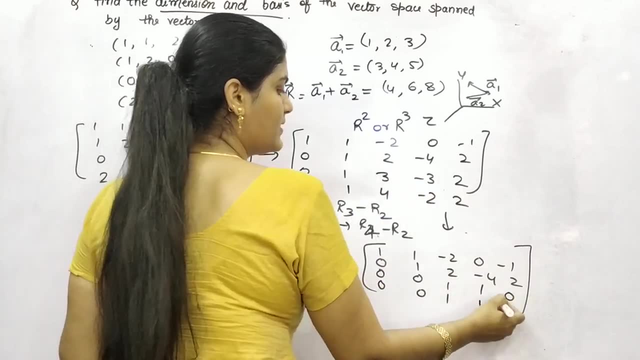 minus 3 plus 4 is 1. 2 minus 2 is 0. 0 minus 0 is 0. 1 minus 1 is 0. 4 minus 3 is 1 minus 2 plus 3 is 1. 2 minus 2 is 0.. 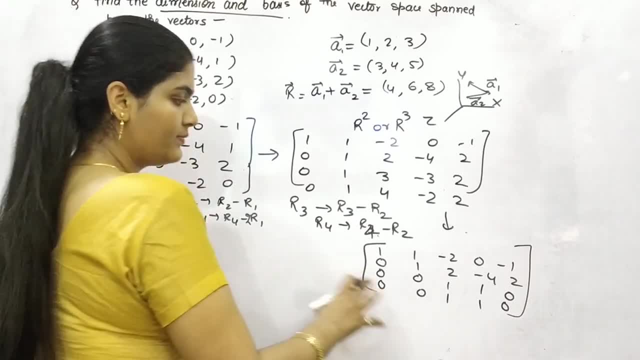 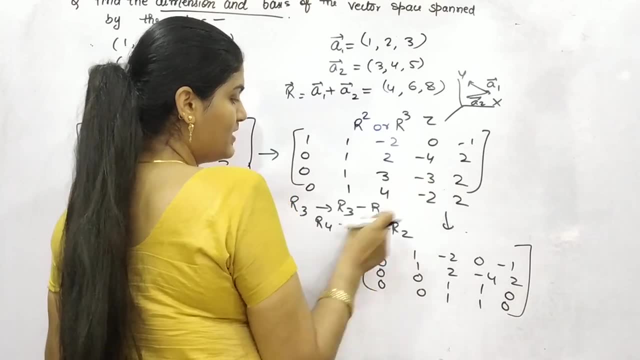 Now, this is what you have got so far. Okay, Four matrices and this is what we have got, Minus 2. Oh, I am really sorry We have to do it from R4 and R2, right, 1 minus 1 is 0. 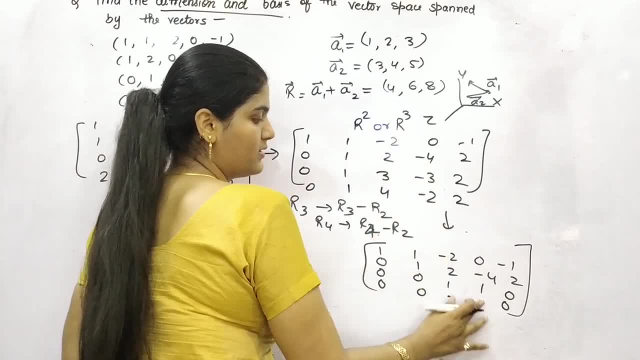 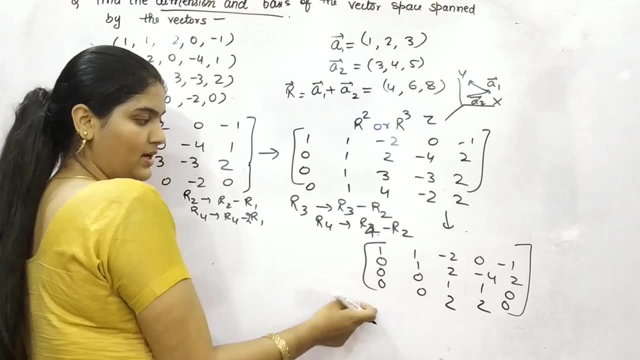 4 minus 2 is 2 minus 2 plus 4 is 2, 2 minus 2 is 0. Initially I applied with R4 and R3, right, But the operation is R4 minus R2.. So this is what you have got. 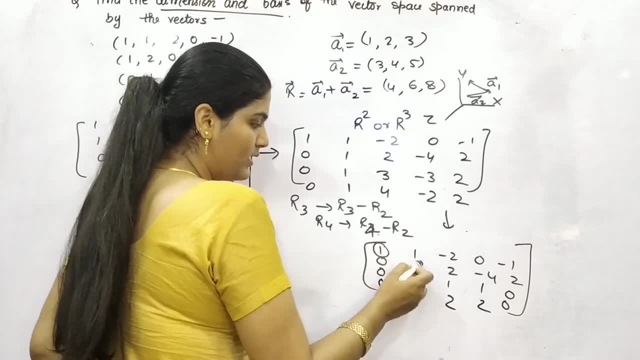 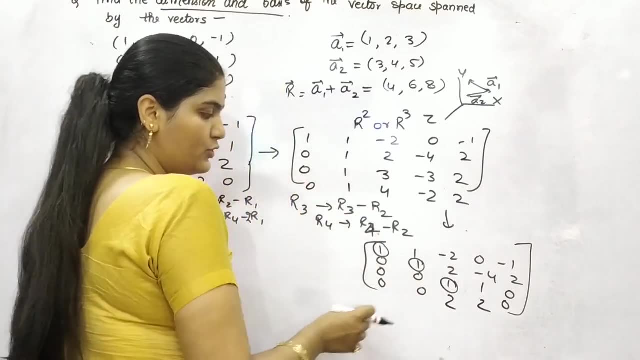 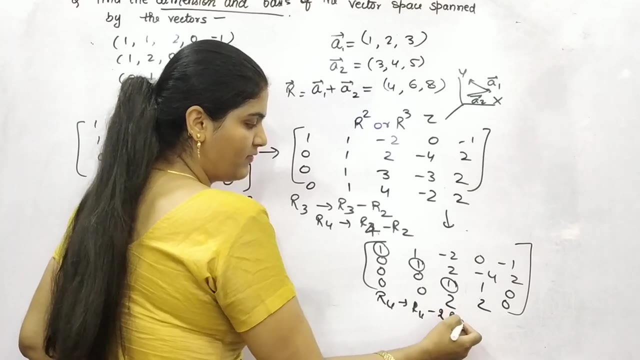 Now find out the pivot points. Pivot means 1, 1, 1. which row is having this? However, you can do one more thing To nullify this 4th row. you can subtract 4 from twice of R3, right? 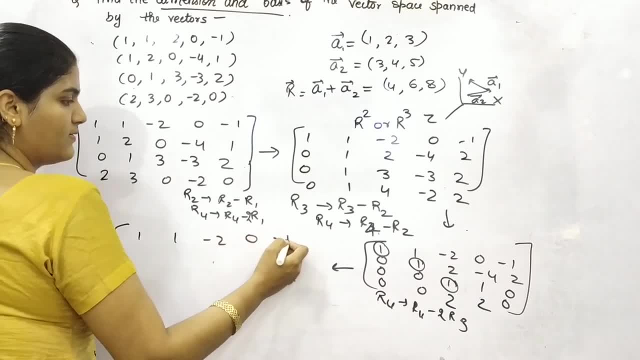 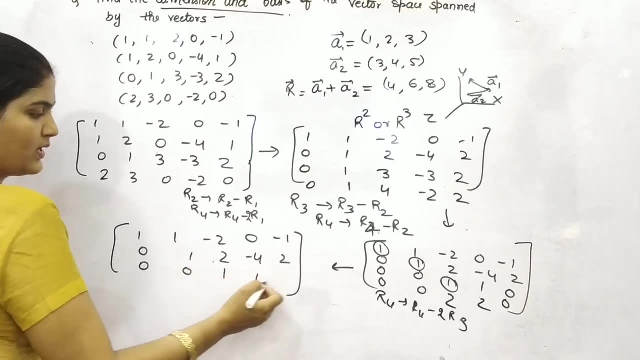 Then what you will get. So first, as it is 0, 1, 2 minus 4, 2, 0, 0, 1, 1, 0. Now for 4th: 2 minus 2 is 0.